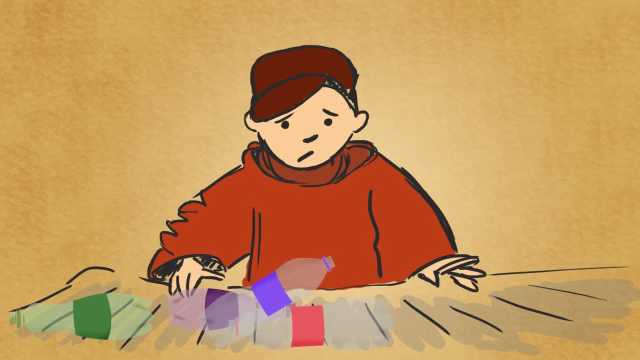 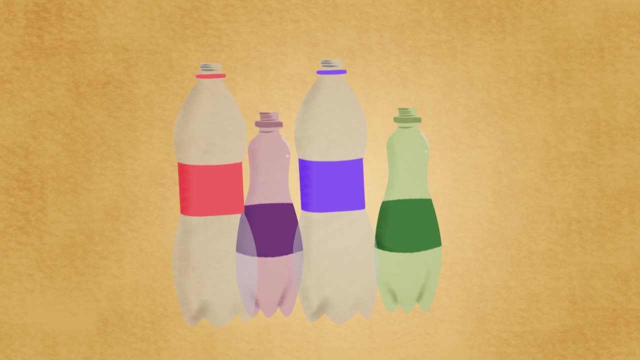 they have to be manually sorted, which is a labour and energy intensive process. Mixed polymers are found in a range of materials so cannot be recycled and are often dumped Once a plastic has been recycled- once it can become downcycled, whereby its quality is decreased- 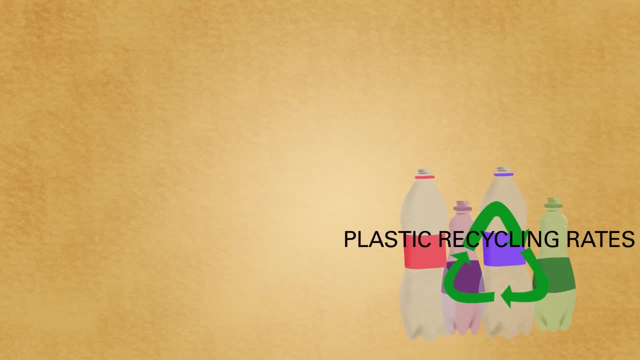 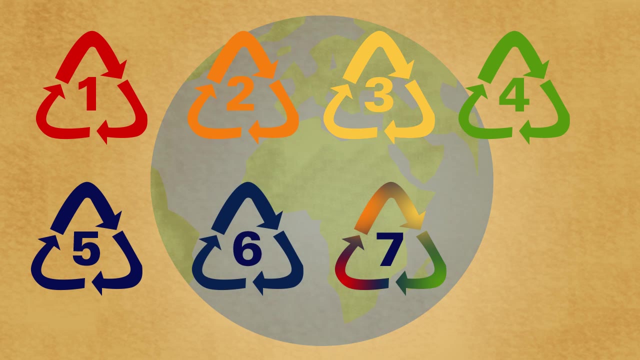 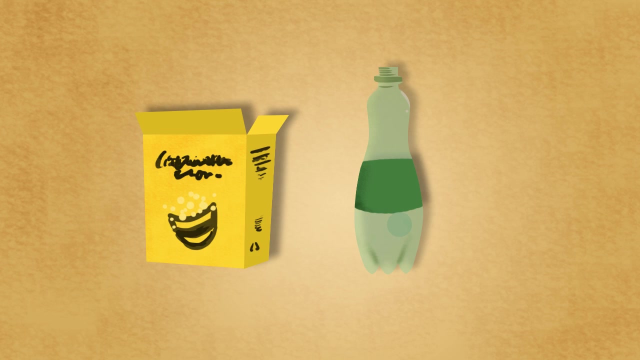 The fact is that plastic recycling rates are far below other recycling rates, but the industry has improved in recent years. Worldwide, seven groups of plastic polymers have been given a plastic identification code that people use for recycling. These you can find on most packaging or plastic materials. Different types of plastics will be recycled by different. 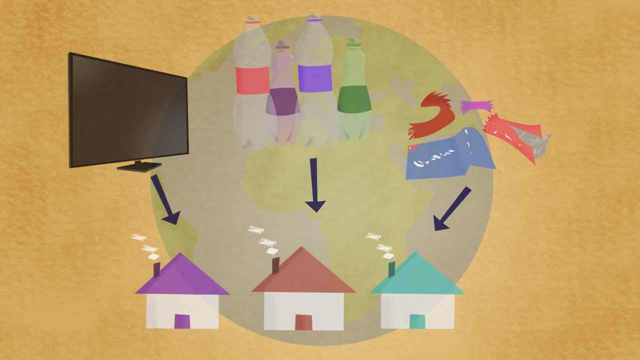 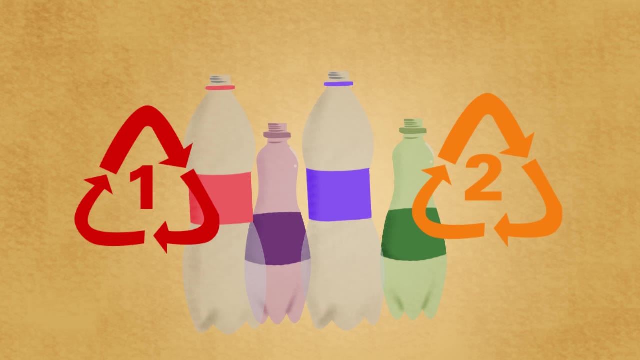 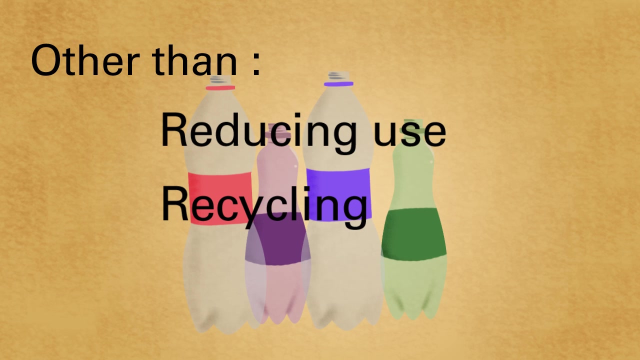 municipalities, even by different countries in some instances. Generally, it's difficult to recycle plastics with numbers one and two. Plastics in these higher numbers are known as rigid plastics. So the disposal of plastics is a tricky one, Other than reducing their use, recycling or reusing them. 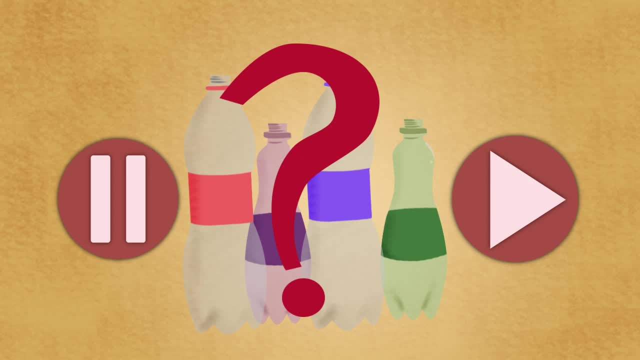 what else do you think might be done to dispose of them? Pause the video and continue when you think you have an idea. If you have any questions, please feel free to ask them in the comments. If you have any questions, please feel free to ask them in the comments. If you have any questions, please feel free to ask them in the comments. 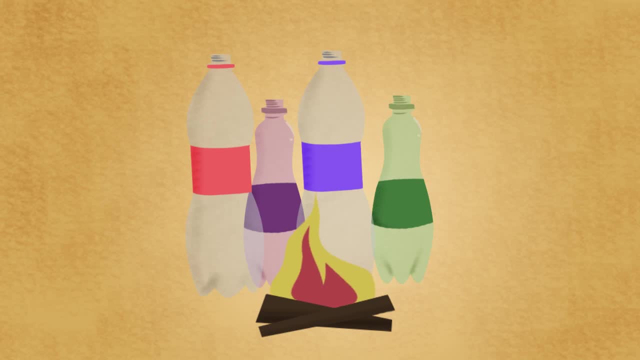 One way is that the plastic can be incinerated or burnt, Whilst this produces useful energy. some plastics contain polymers that are halogenated. When these polymers are burnt, for instance PVC, toxic fumes like hydrochloric acid are released. This can cause severe 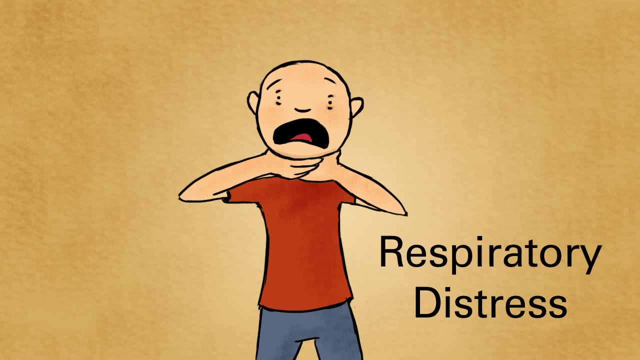 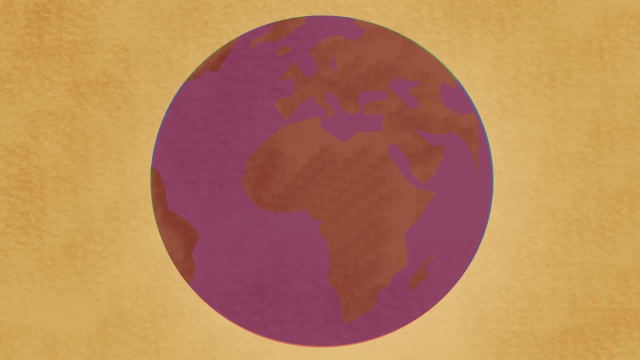 respiratory distress, and so is hugely problematic. In addition, burning of polymers produces CO2, the greenhouse gas, and so can carbon dioxide. This can cause a lot of damage to the environment. In addition, burning of polymers produces CO2, the greenhouse gas, and so can carbon dioxide. This can cause a lot of damage to the environment. 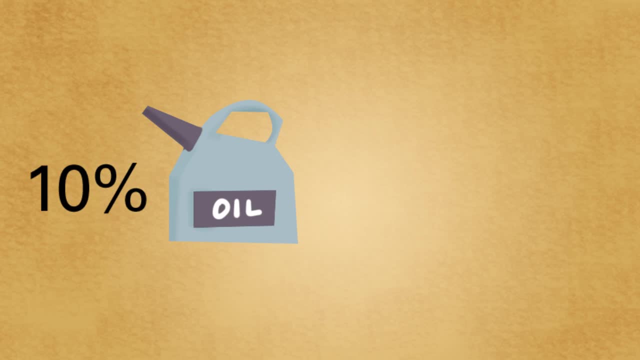 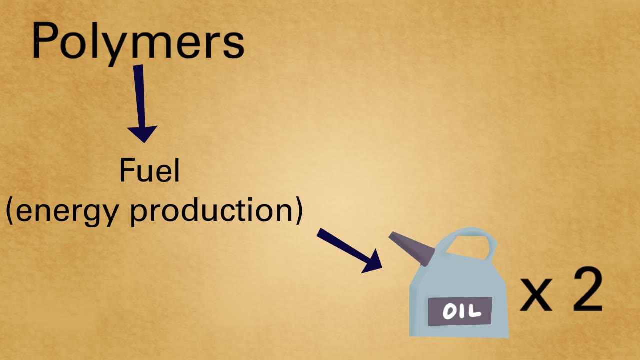 This is because about 10% of the Christchurch Sea's oil is used as petrochemicals. If we then use the polymers again as a a fuel for energy production, then at least we are using the oil twice. There is no time to feelsize. This could affect the quality. of any of the plastics. But now what we have to rethink that it might be possible to use bioplastics as a solution for Ultimately, how would you think bioplastic becomes bioplastics? mulядar, i e Matthew 봐 start with answer. 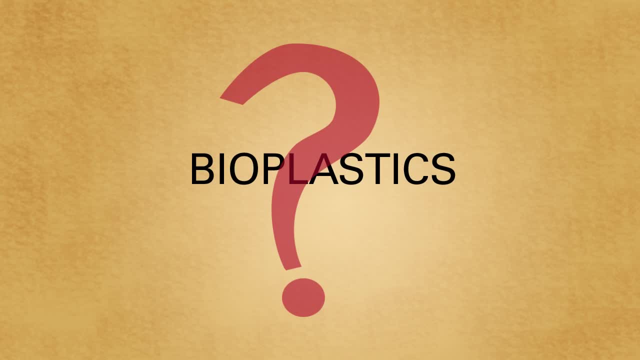 You may have heard the idea of using bioplastics as a solution, But these too can have problems. What do you think a bioplastic is? Beyond the term bioplastic, might you have the answer is: Pause the video and resume when you have an answer. A bioplastic is a biodegradable plastic.